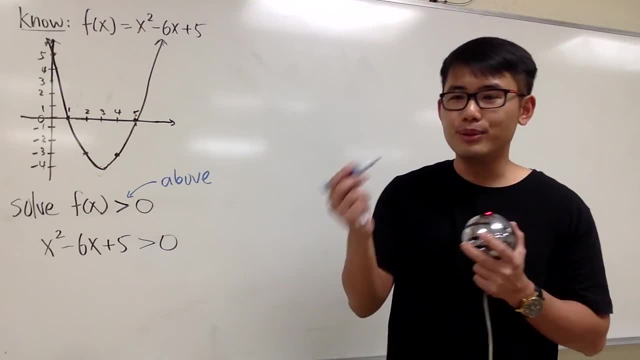 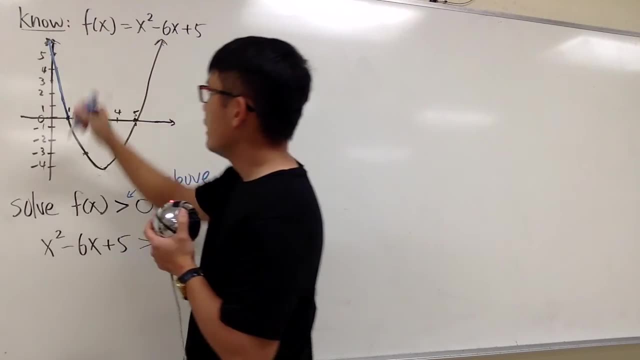 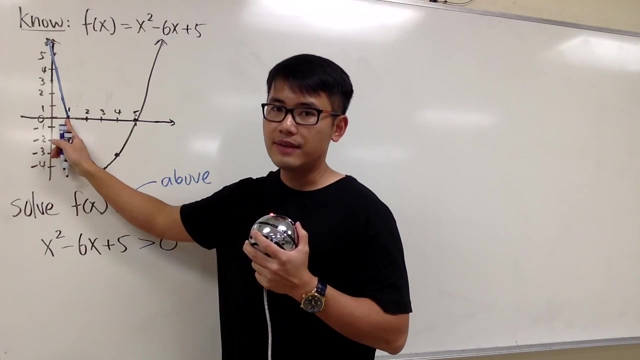 And let me color these two portions for you guys in blue. So this part of the graph, it's being above 0, and let's write down the answer for this. And we are looking for the x values. This right here is 1 for the x value, but we are looking for 1 and anything to the left, right. 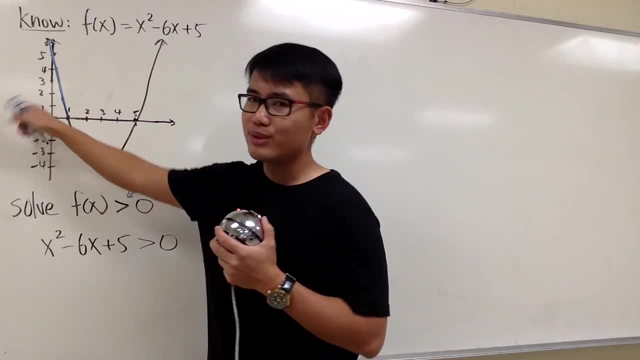 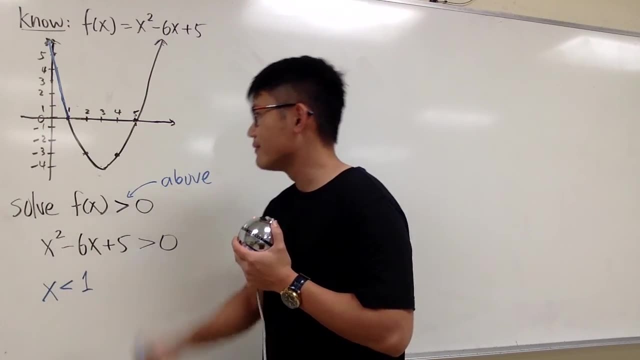 So you see, we have the 1 with the 0, negative numbers, and so on, so on, so on. So the first part of the answer will be: x is going to be less than 1.. 1 and less. 1 and less. 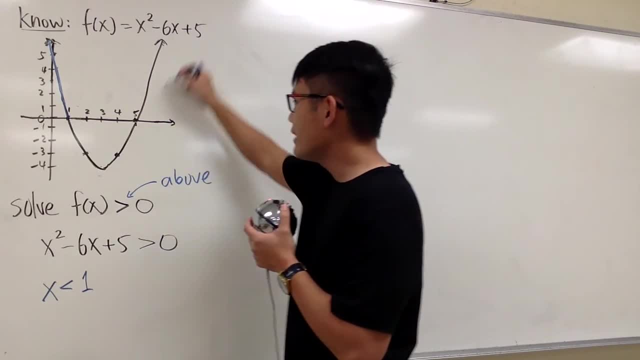 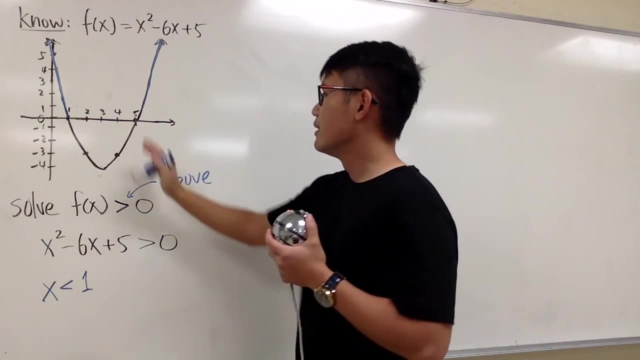 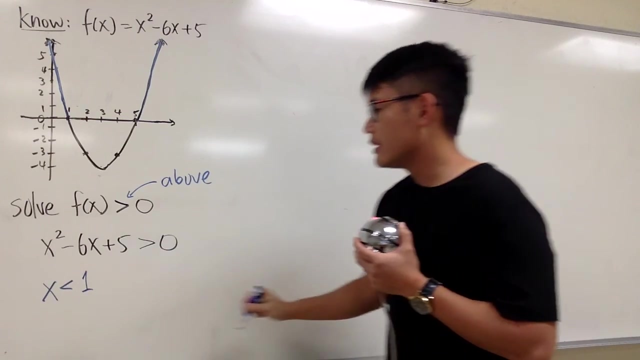 Where else, though, We have the second one right here, from 5,- and you see, the graph is being above as well, And the x values are going from 5 and bigger, 5 and bigger, And toward the right. So this is the first part: x or less than 1, right. 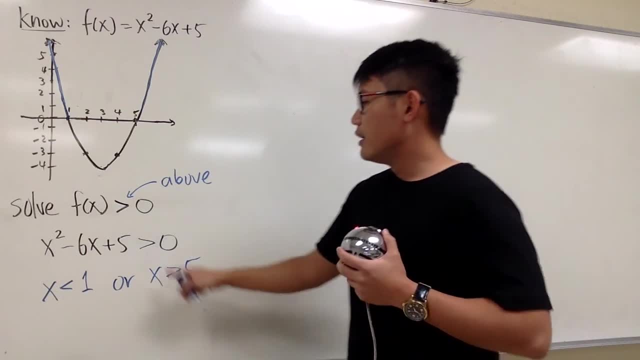 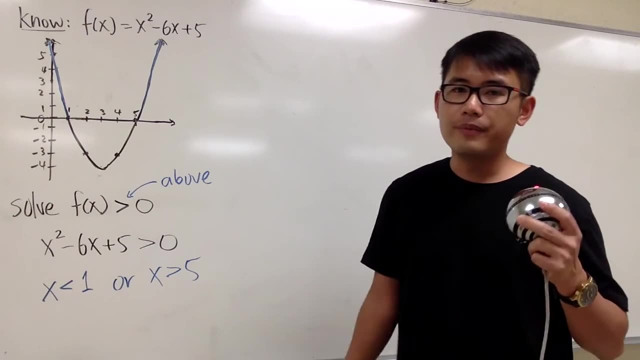 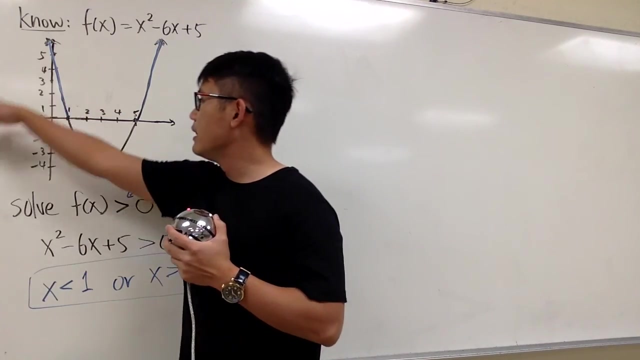 Or the second part is: x is greater than 5. Originally we just have a greater than. there was no equal sign, so we don't have equal signs right here and right here either, And hopefully you guys will be convinced that this right here is the correct answer, because we have the less than part right. 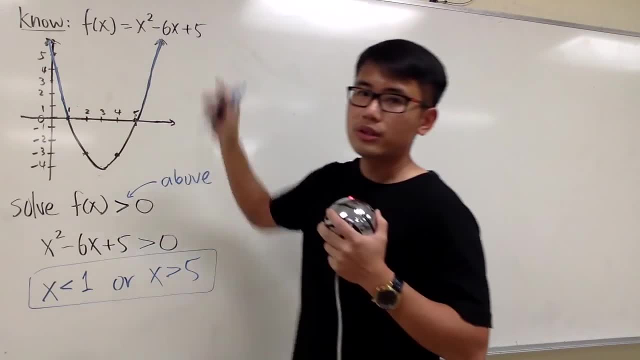 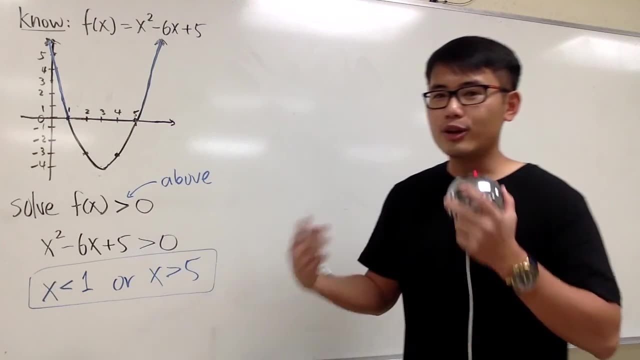 The x is less than 1, and we have the x is greater than 5.. So we have two portions, two pieces, And we're done. No problem with this. However, what if, by doing some algebra work without the graph, can I do that? 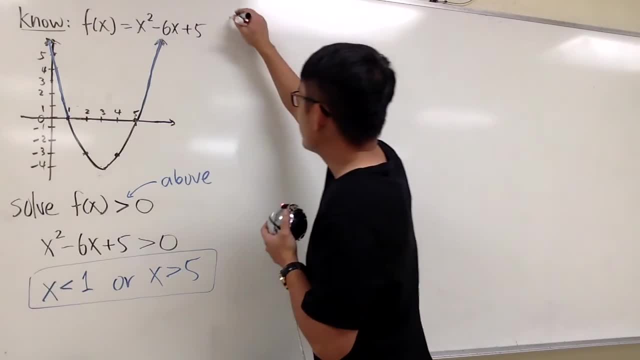 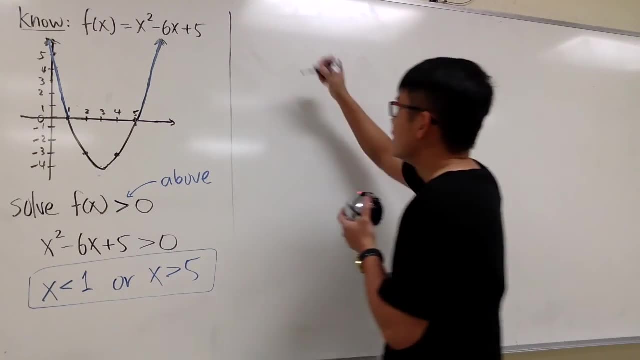 Well, let me show you what can we do. So now, right here, I'm just going to demonstrate how we can do this inequality without using the graph. Suppose I want to solve from scratch that x squared minus 6x. 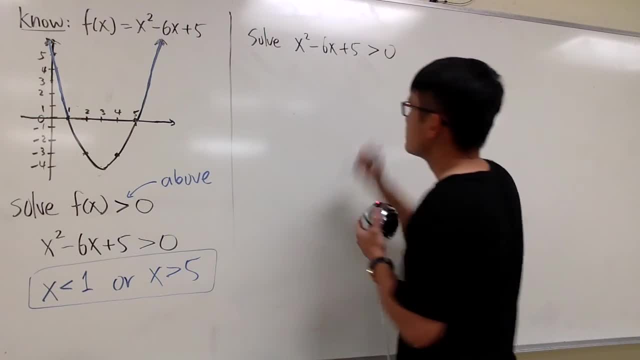 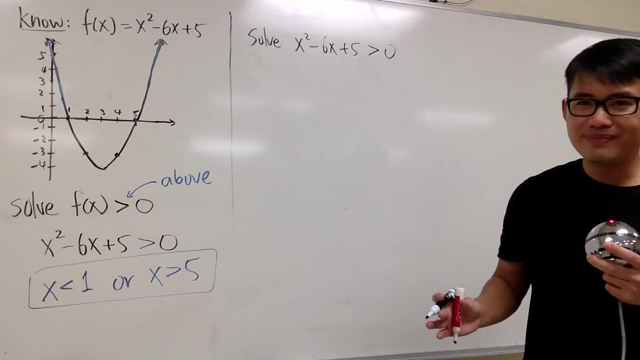 6x plus 5 is greater than 0.. I'm going to demonstrate what is wrong- and don't do it this way- And you will see why it is wrong. okay, So I'm going to just show you guys this right here. it's going to be the wrong way to do it. 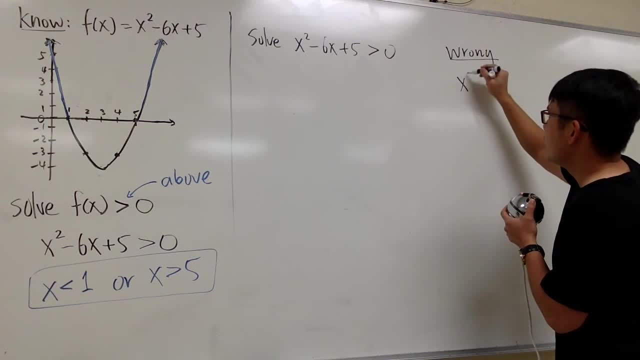 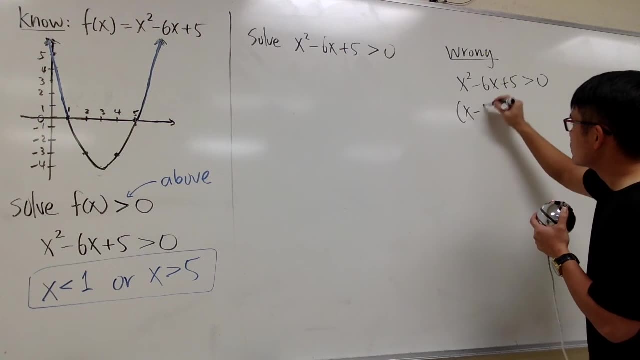 Don't ever do this. Let me write that down again: When you have x squared minus 6x plus 5 is greater than 0,. yes, we can factor this out. we can get x minus 1 times x minus 5.. 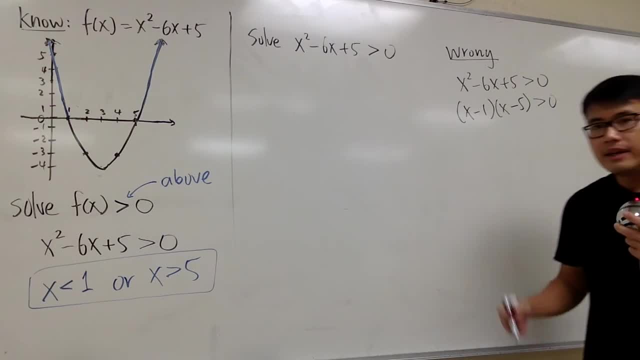 That's the factor for this, and this is greater than 0,, isn't it? And you see that we have the 0 on the right-hand side, but don't get too excited and just put down. hey, let me put this down. 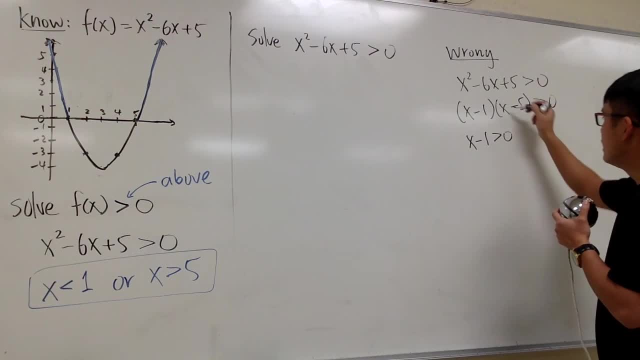 x minus 1, and write that down greater than 0, and let me write this down: Or x minus 5, and put that down greater than 0. And I'm just going to add 1 on both sides. so it seems that we have x is greater than 1.. 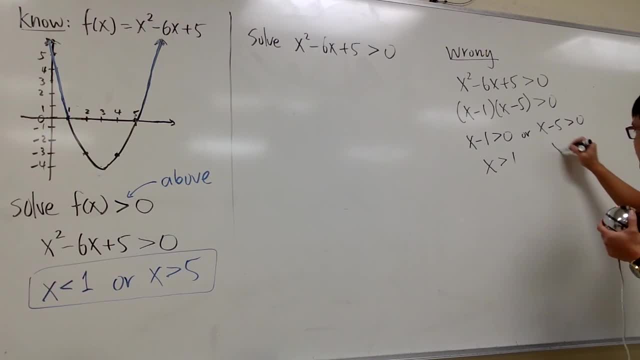 And let me add 5 on both sides, And it seems that we have: x is greater than 5.. It seems that this is okay. But look at this, look at that. What's the difference? Well, this portion is okay. x is greater than 5.. 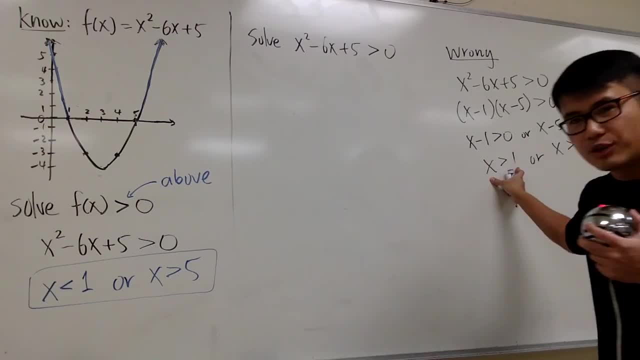 However, this is x greater than 1, which is incorrect. This is wrong Because we're supposed to get: x is less than 1.. And if you just do it like this, there is no indication on why we should switch the equation. 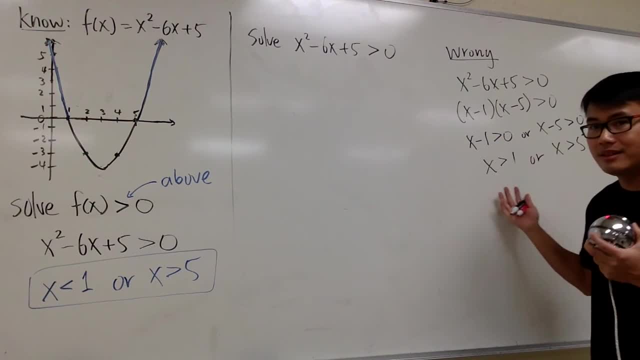 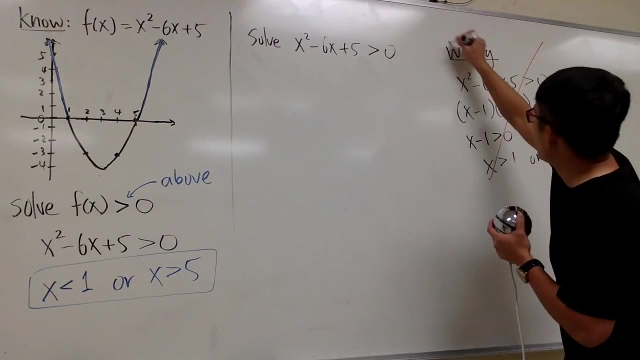 There's no indication on why we should switch the inequality symbol right. There's no indication on why we should switch the inequality symbol. So, seriously, don't ever do it like this, And this is just dangerous and not correct. And now let me show you guys the way to do it. 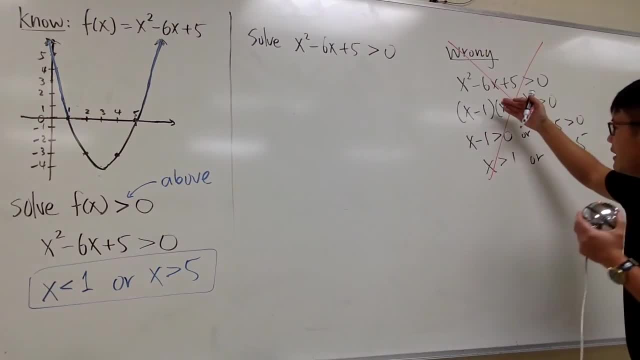 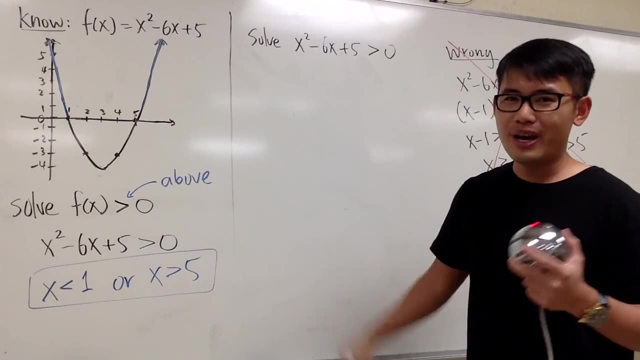 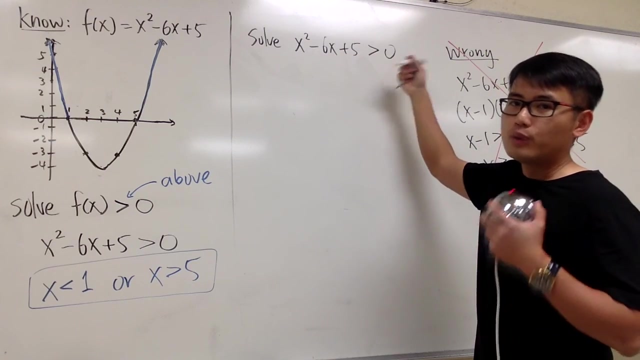 And once again, the trouble is that we don't have any indication on why we should switch the inequality symbol. You can use the graph or you can do it this way, So pay attention to this. First of all, make sure that the right-hand side is equal to 0, which it is. 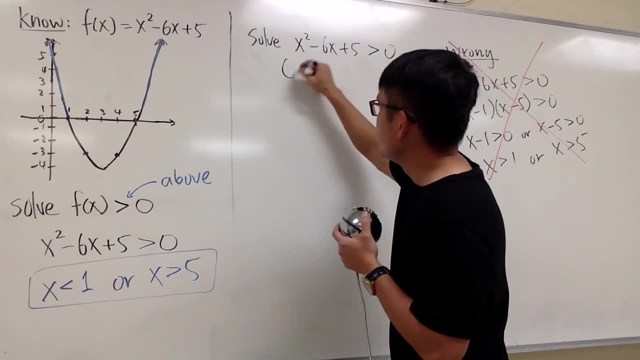 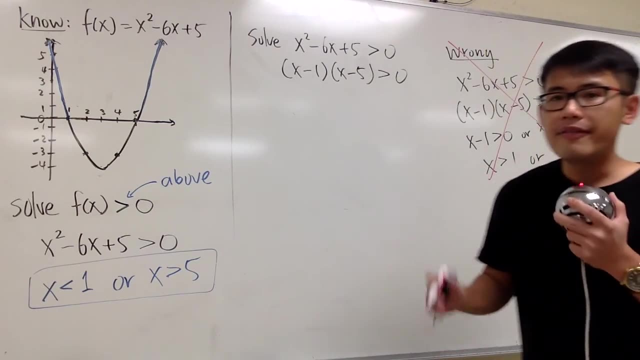 That's good, And I'm going to factor this out as well. And we know it's going to be x minus 1 times x minus 5.. And let me write that down as well: It's greater than 0.. And now we have to find out the numbers that we care. 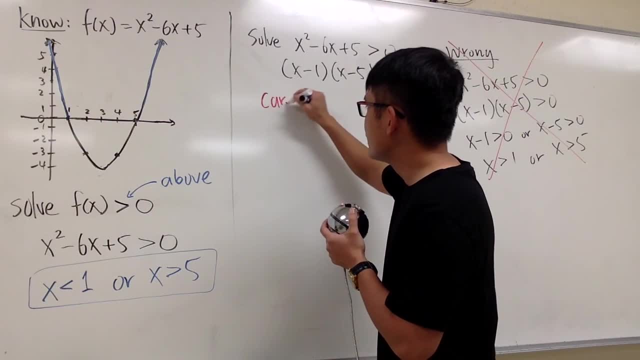 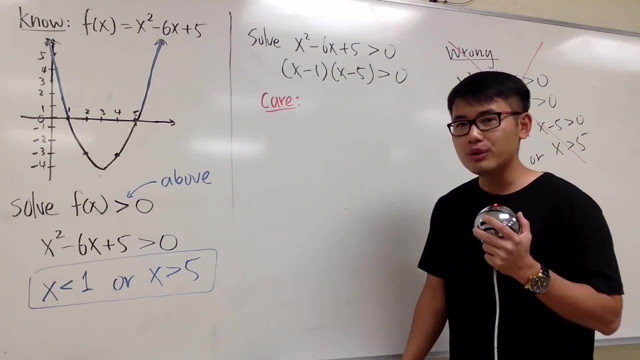 And let me write down the word care, Because when I write down the word care, you know you have to care about these two numbers. And let me tell you, guys, this: We care about two numbers and those numbers are 1 and 5.. 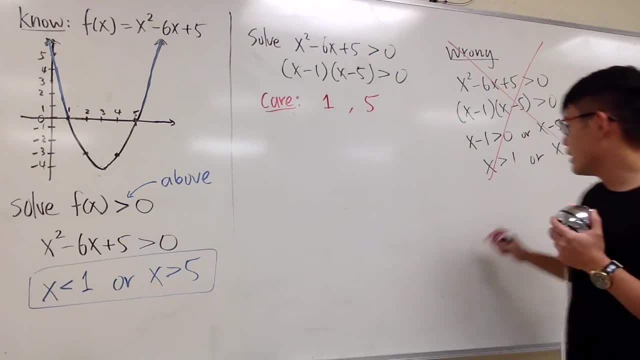 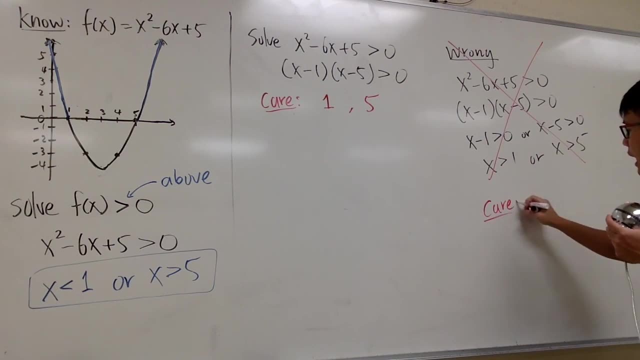 How do we know? Well, you can do it this way. The first number that we care is- you write this down right: x minus 1.. So this is: we care about how we can get x minus 1 to be 0.. 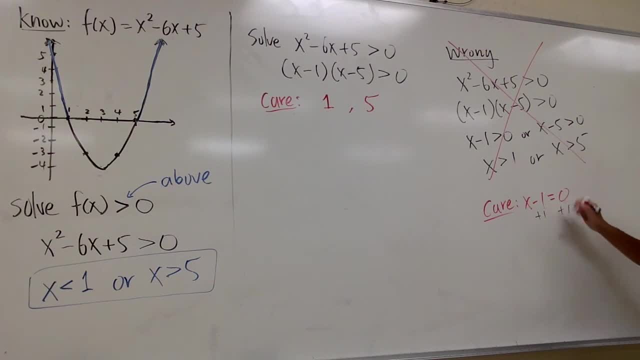 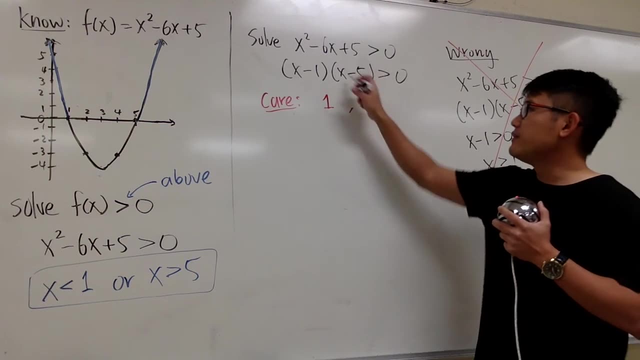 And I can add one on both sides. So you know, the first number that you care is x is equal to 1.. And the second number is: you set this factor, which is x minus 5 equal to 0. And then, of course, we can add 5 on both sides. 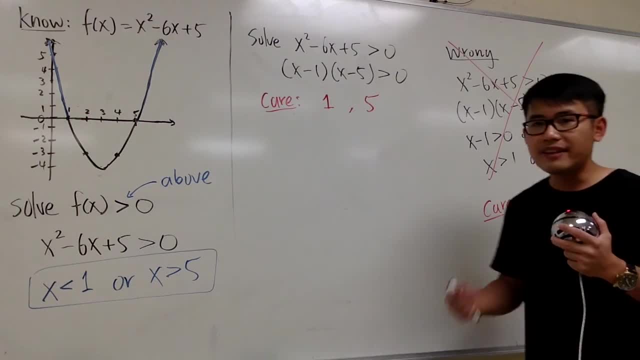 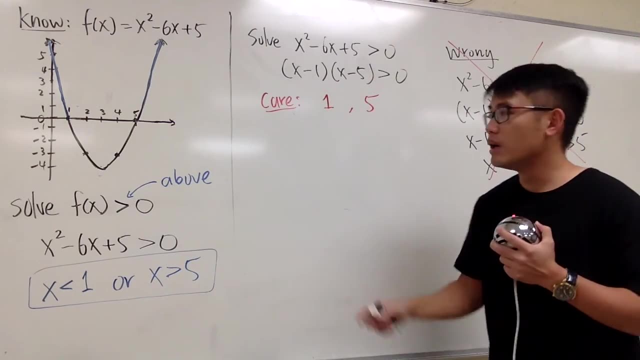 So the second number is: x is equal to 5.. These are the numbers that we care. okay, So 1 and 5.. You can just look at this factor and write it down, But be careful how you can make this factor equal to 0.. 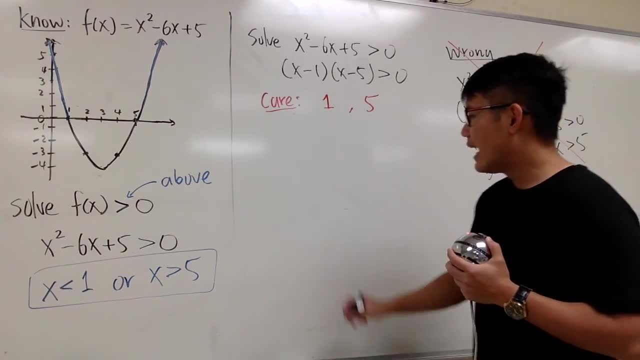 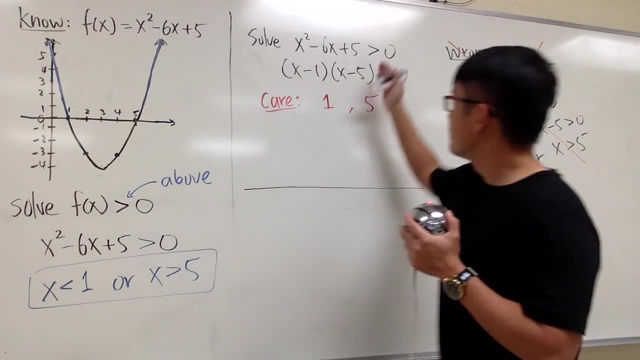 These are the two numbers that we care and this is how we're going to finish it. I'm going to draw a number line And the reason is because, remember, whenever we have an inequality, we have the inequality that will associate with the graph. 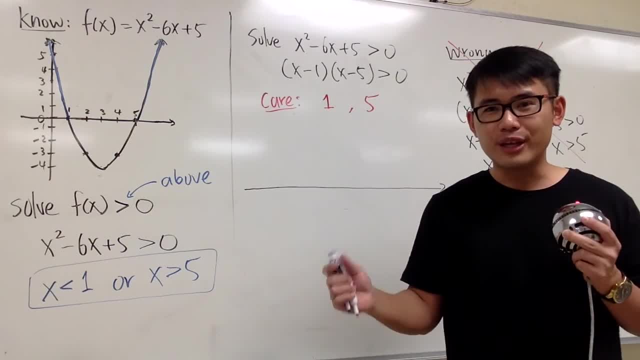 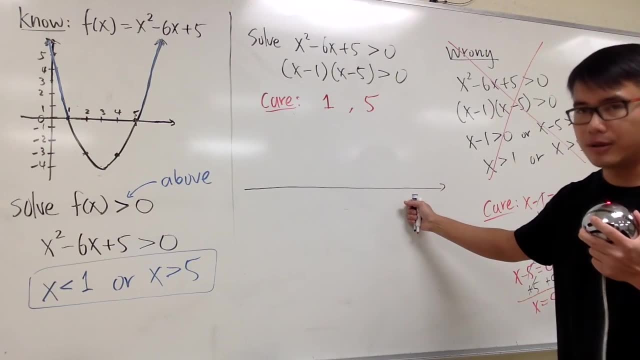 and we can also associate that with the interval notation- All of the three things that I just mentioned. they are connected with each other. Let's use the graph to help us out. On the graph, I'm going to put down the two numbers that I care. 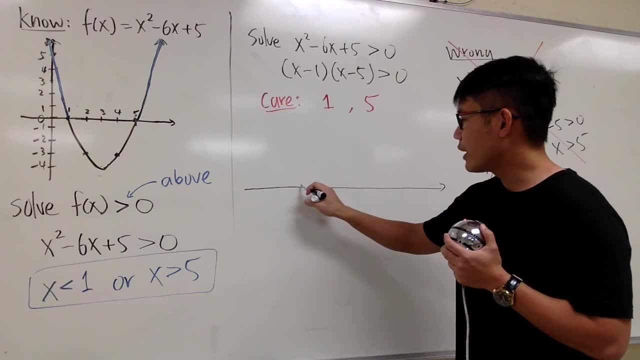 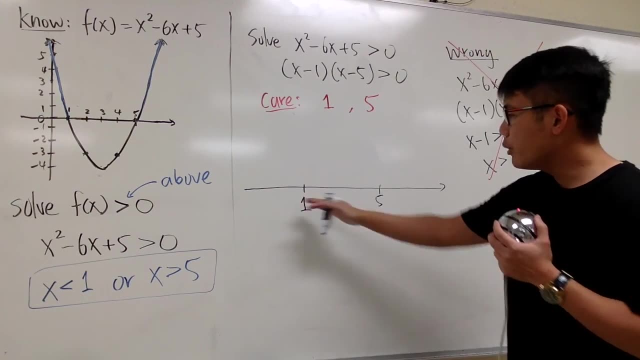 which is 1 and 5.. And put down 1 right here because 1 is smaller, And then put down 5 right here because 5 is bigger, right? So be sure you label them on the number line correctly as well. 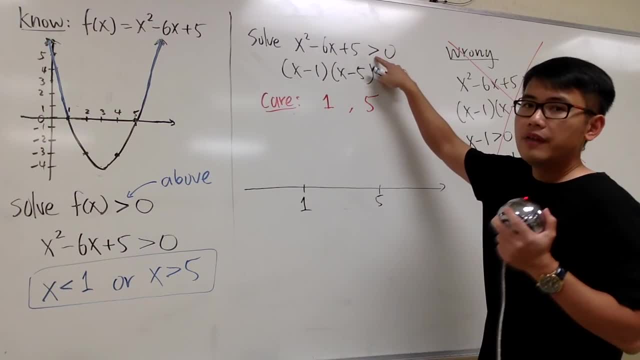 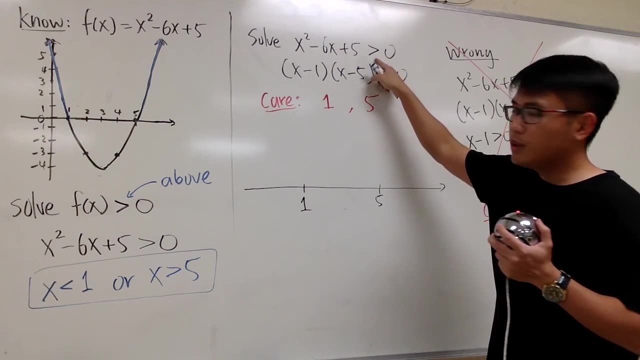 And let's refer back to the original inequality. This is just a greater than symbol. There's no equal sign. right For the two numbers that I care, because there's no equal sign, even though I care about them, but I don't want to have them. 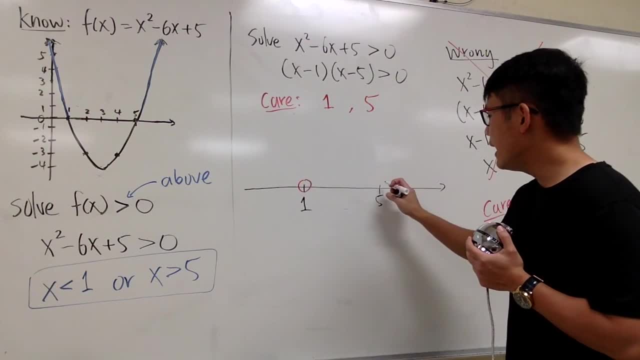 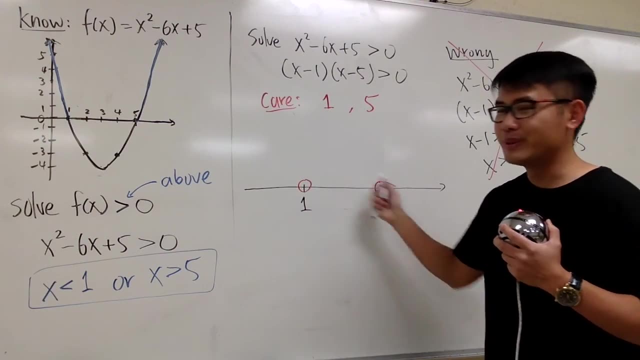 With that being said, I'm going to put down an open circle here and an open circle here Once again. we care about these two numbers, but we don't want to include them just because there was no equal sign. If there was an equal sign, 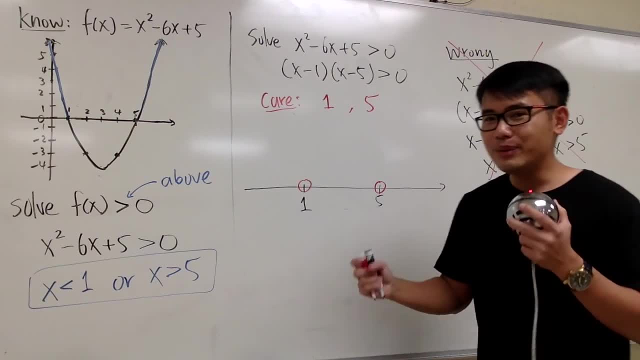 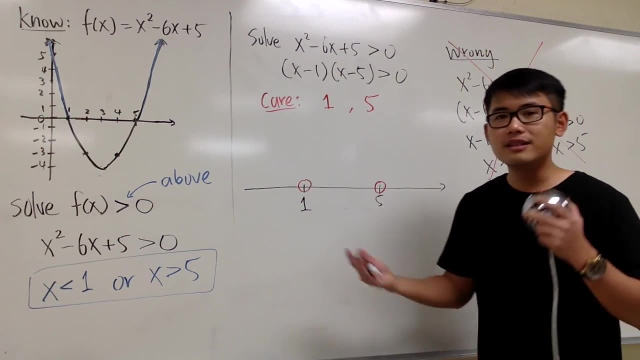 I would fill in with a closed circle. Anyways, and now you see, on the number line we have three intervals: First one, second one and the third one. And this is how we're going to do it For the first one. 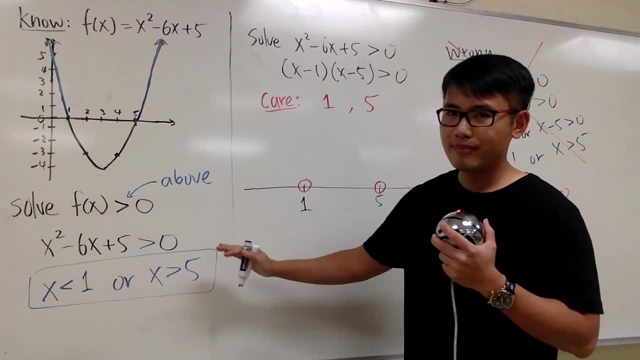 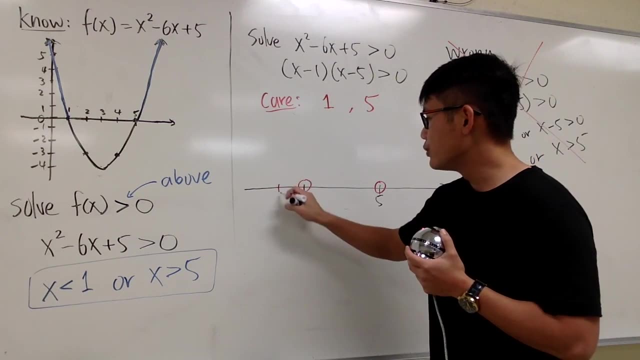 I'm going to think about a number less than 1.. So we can use 0,, we can use negative 5,, we can use negative 22, up to you, But I'm just going to use 0, and this is going to be the test value. 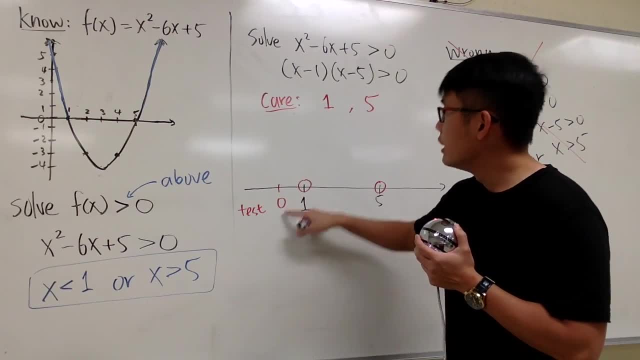 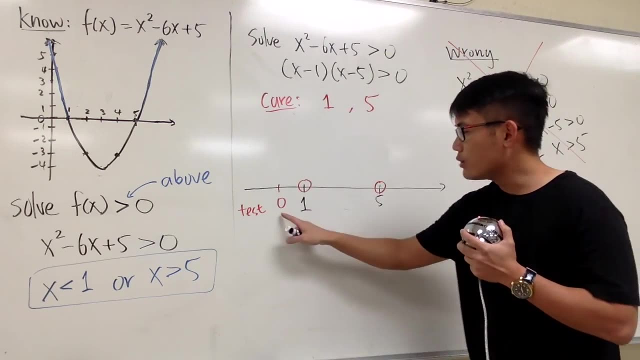 And what we're going to do is I'm going to plug in 0 back to the factory form. It's easier. You can also plug in 0 into the original- Up to you, seriously. But I want to plug in 0 into the factory form. 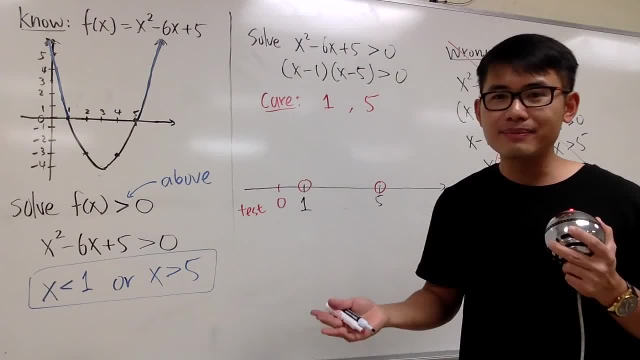 And then work it out to see if we end up with a true statement or not. If it's true, I will call it, If it's not, leave it. So that's it, Plugging 0 into this x and that x. 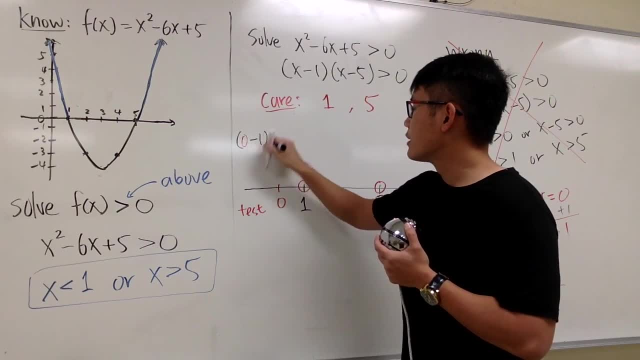 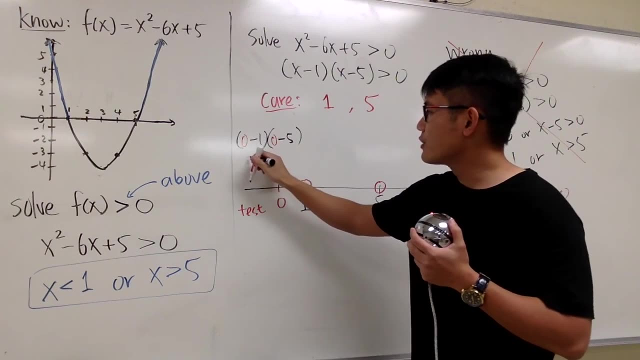 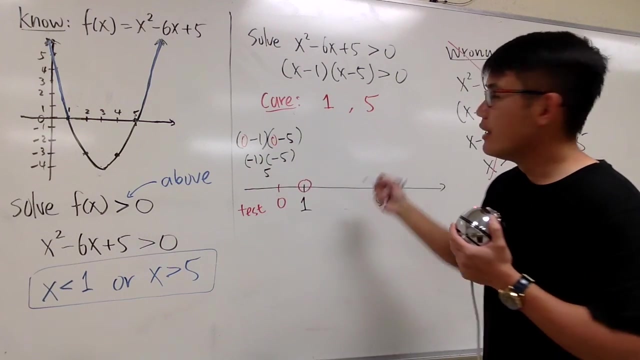 we will have 0 minus 1 times 0 minus 5.. And let's work this out first. This right here is going to be negative 1 times negative 5.. Well, negative 1 times negative 5 is positive 5.. 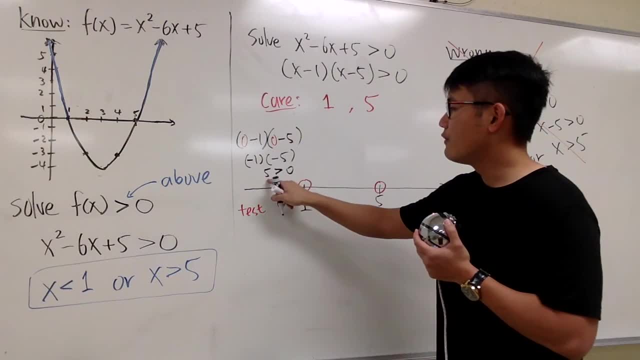 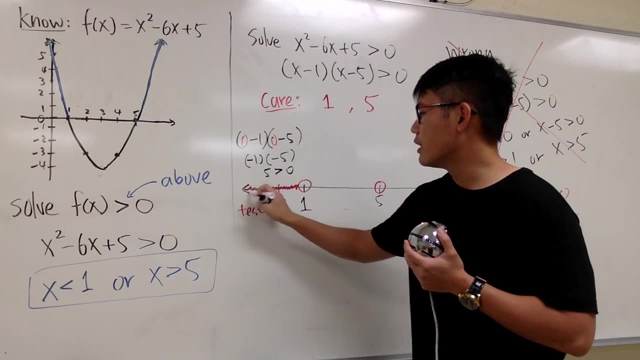 And check it. We are trying to see if something is greater than 0.. 5 is greater than 0. Of course It's true, And you are just going to color this portion. It's going to be 1 and less. 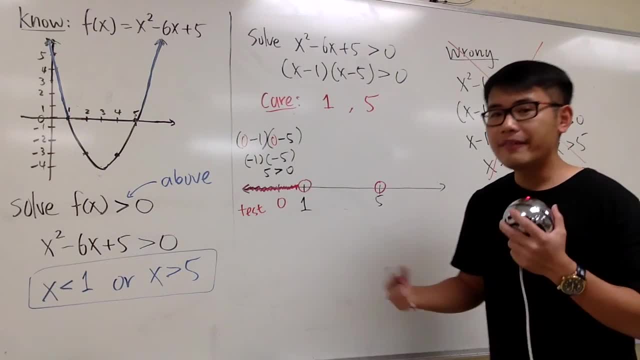 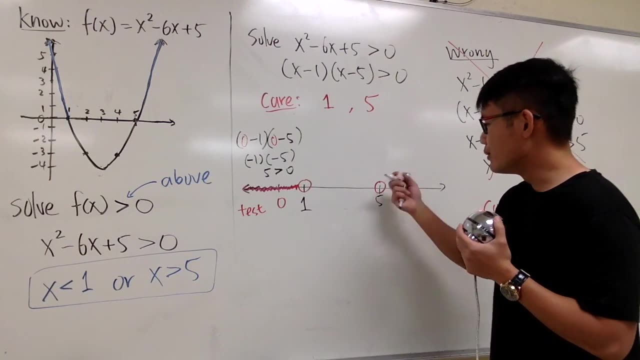 1 and less. 1 and less. Okay, And now pick a number between 1 and 5. You can use 2.. You can use 3.. Up to you And just to you know. just to emphasize. 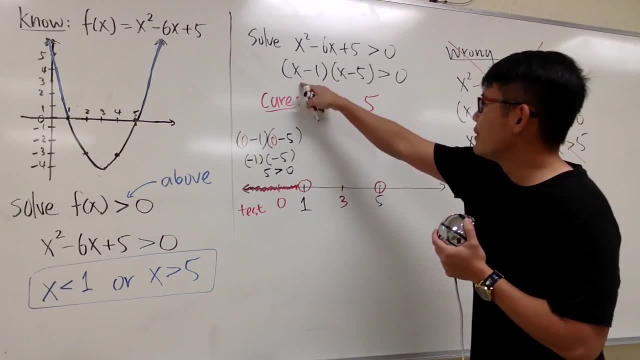 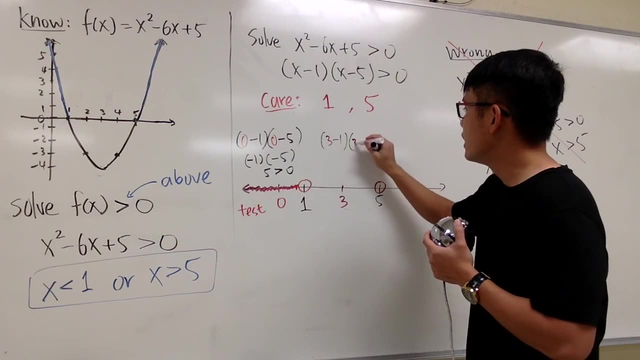 you can use any number. Let me just use 3. Plug in 3 into here and here and work it out. So that's it. We will have 3 minus 1 times 3 minus 5. And we know 3 minus 1 is what. 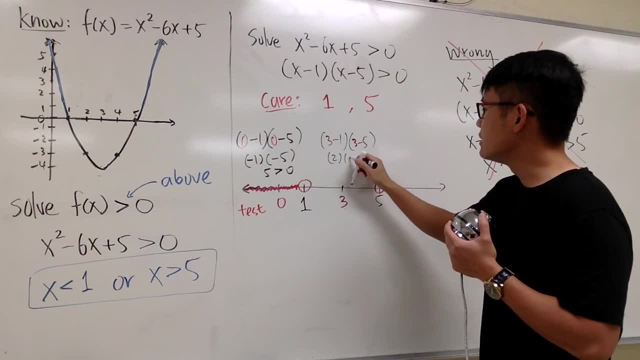 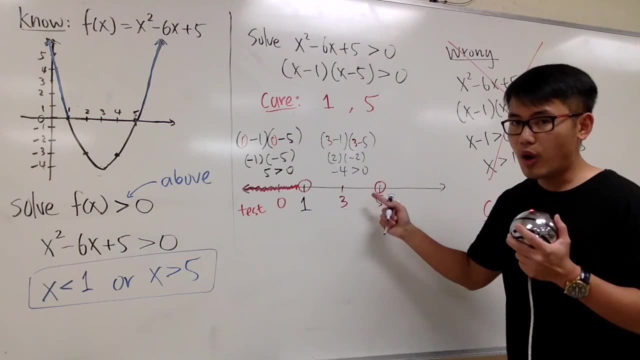 2, right And then 3 minus 5 is negative 2.. 2 times negative 2 is negative 4. Is this greater than 0?? No, Negative 4 is not greater than 0. So this is the false region. 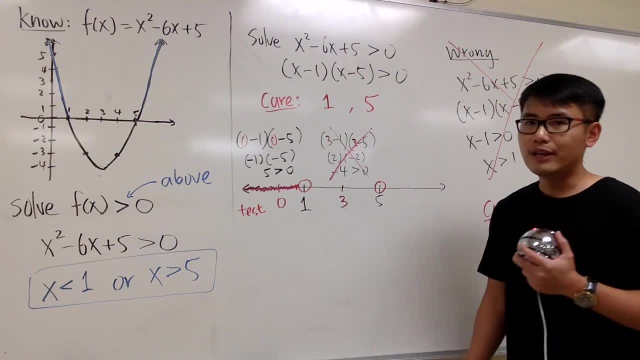 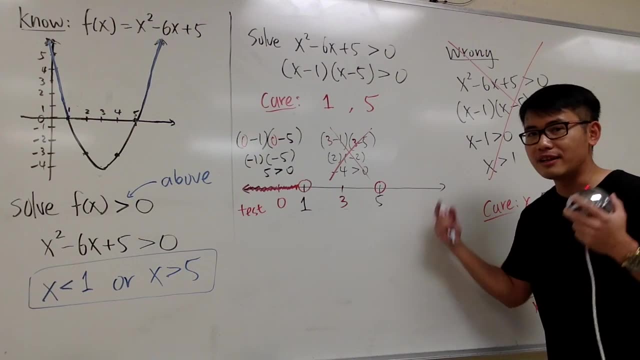 You are not going to include this region- Don't color this in- And you just are going to repeat the next one. Pick a number that's bigger than 5.. 6,, 7,, 8,, 9,, 10.. 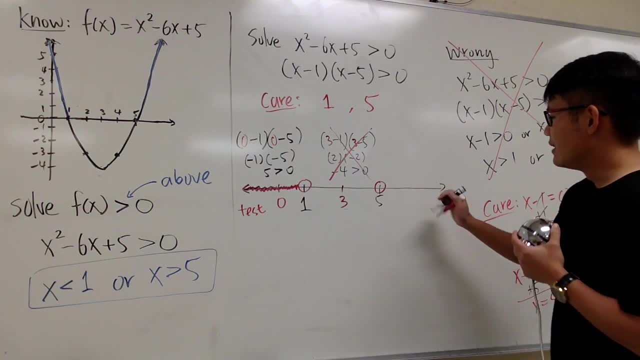 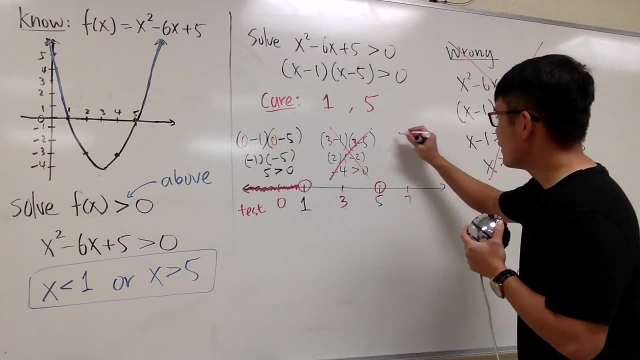 6.5, 5.1.. Up to you, And let me just say that I want to use 7.. Just to emphasize, you can use any number. Let me use 7.. Plug in 7 into here, So we have 7 minus 1. 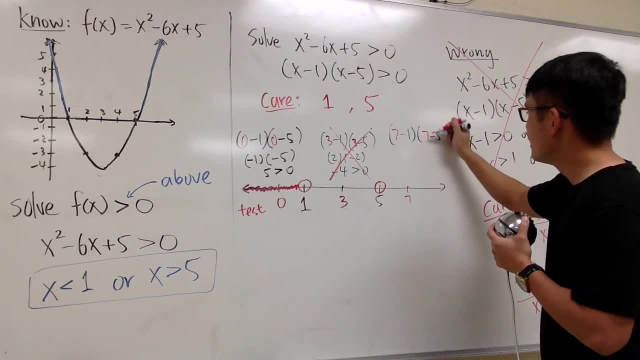 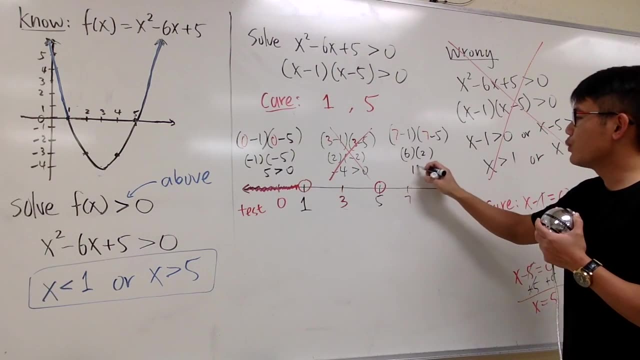 times 7 minus 5.. And let's just work it out: 7 minus 1 is 6 times 7 minus 5 is 2.. 6 times 2 is 12.. 12 is of course bigger than 0.. 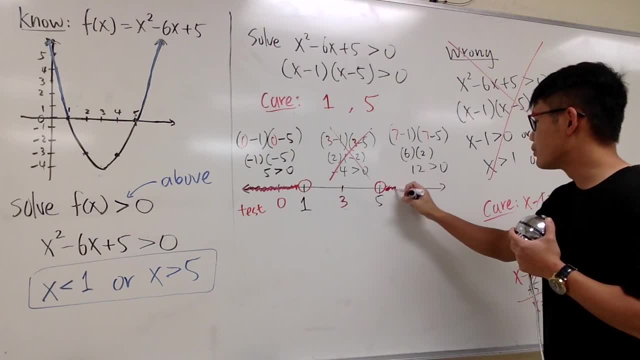 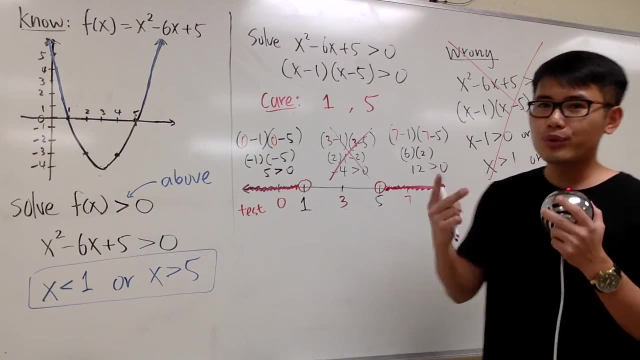 And that means I'm going to color this portion, I'm going to color this section as well. This interval is also going to be part of the answer And, as you can see, we have two parts Right: The first interval and the second interval. 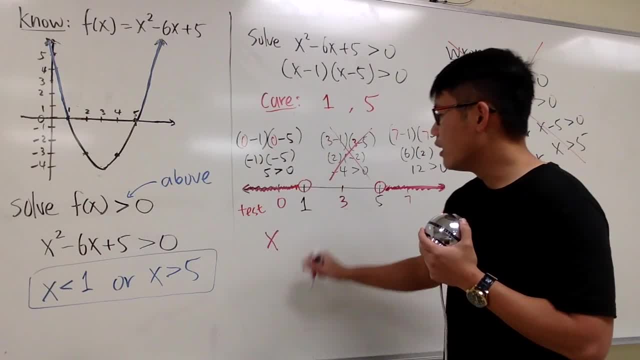 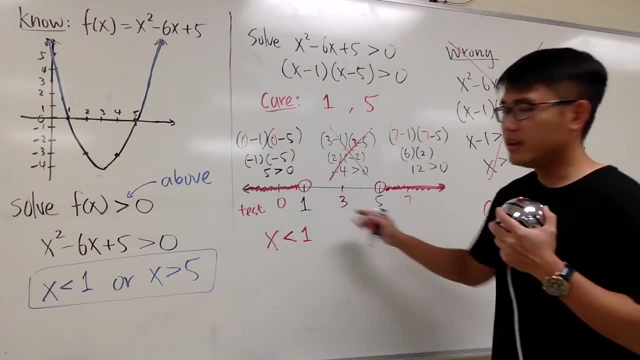 This right. here is what This is: x values less than 1.. Right, I'm not using the 0 or the 3 or the 7.. These were the test values And I care about the 1 and the 5.. 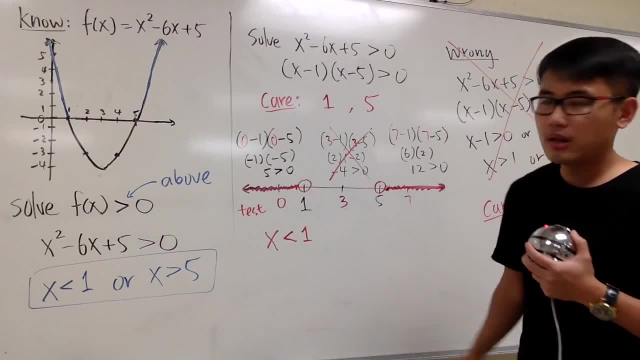 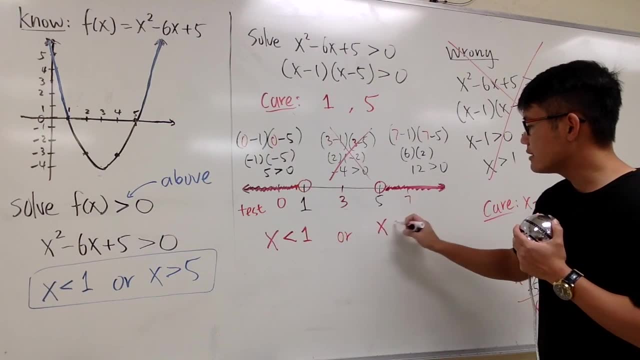 It's 1 and less, x is less than 1.. And we have the second interval here And we have the third interval as well. So I put on or, and we have 5 or more Right, So we can write this down. 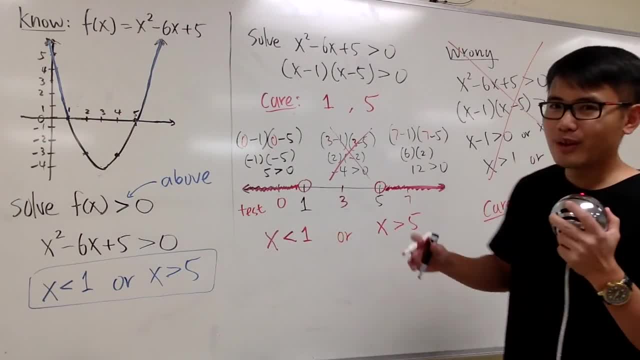 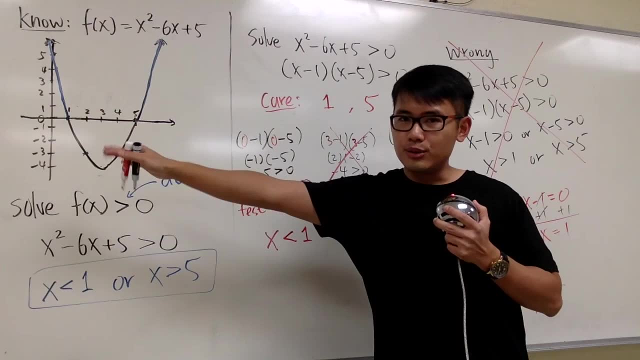 as x is greater than 5.. And now you see, this is the same as that. At the end we can also write this down in interval notation For the interval notation for the first interval. this is all the way going to the left. 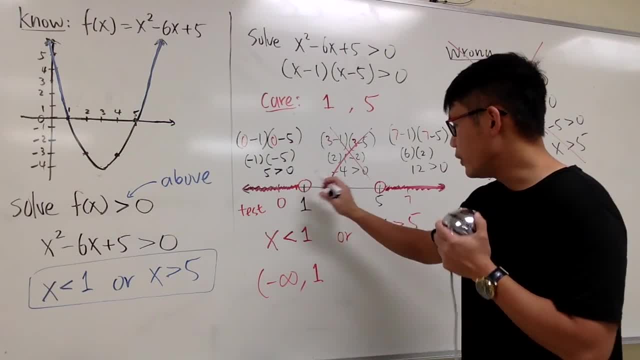 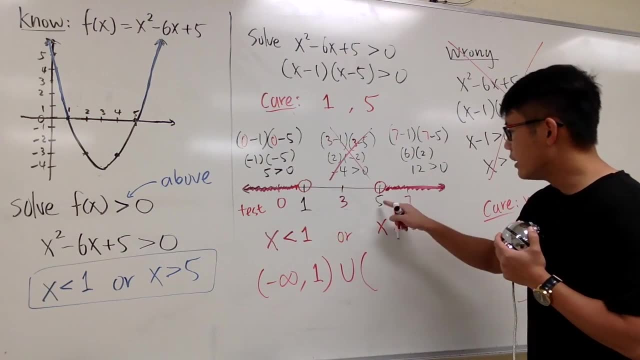 Right, So it's negative infinity And use the parentheses for that. And we have the union for the or, because we have the second piece. The second piece is not including the 5. And then you go all the way to the right. 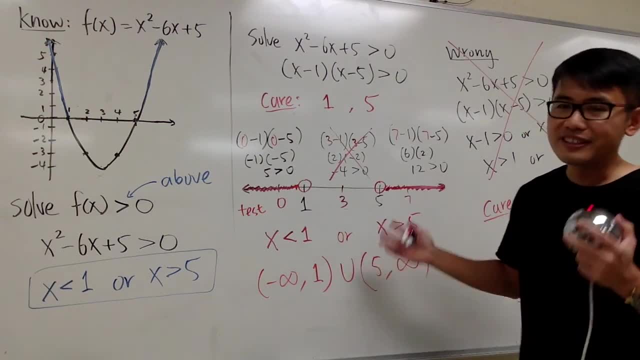 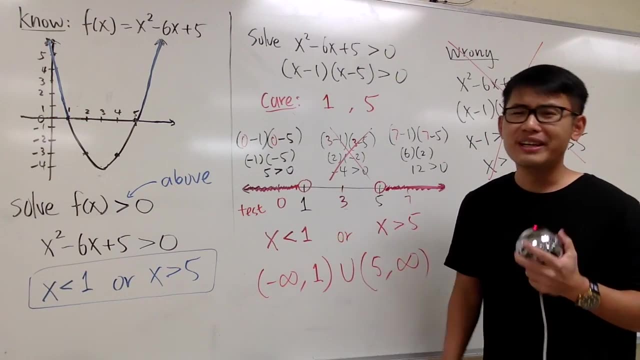 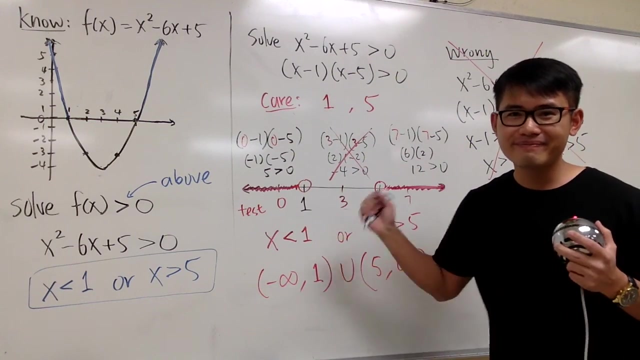 So it's 5 to infinity And I'll close that. So this is how you can do it without the graph, And this is the safest way to make this work. And seriously, I know this is tricky, But once you get a hang of this,